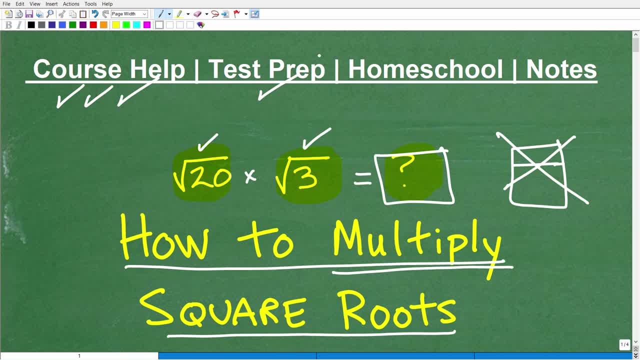 that has a math section on it. I'm talking about things like the GED, SAT, ACT, maybe a college entrance exam or college placement or teacher certification exam. There's a ton of tests out there that people have to take with math sections on it. I can help you prepare and pass those exams. 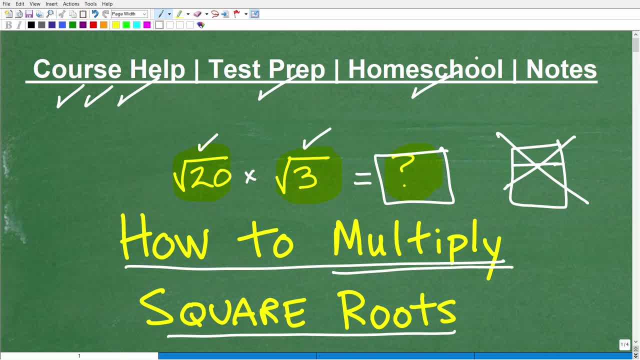 If you homeschool, you've got to check out my homeschool math courses. They were just recently voted number one for middle and high school mathematics by a major homeschool publication, And if you need some math notes, I'm going to leave links to my math notes in the description. 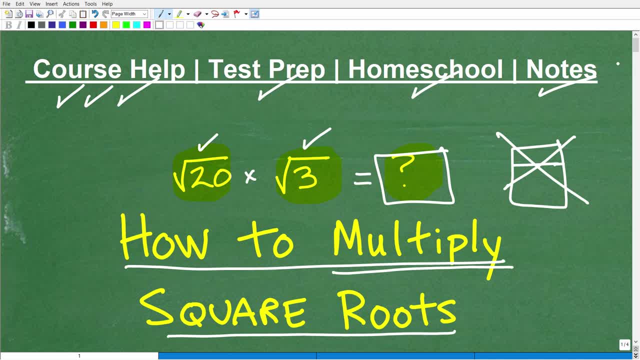 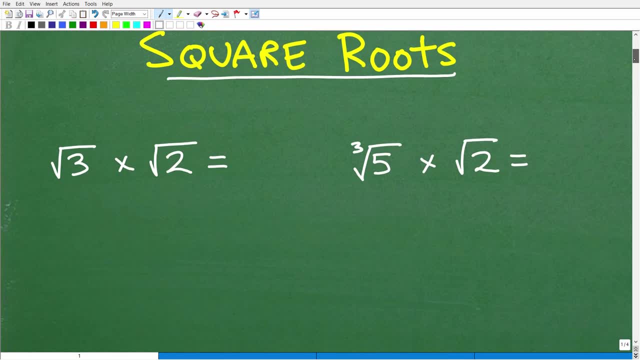 of this video, Okay, so let's get going here and learn how to multiply square roots, And I'm going to deal with this problem here in just one second. I'm not going to forget about that, but let's start this off pretty easy. Okay, All right. So here we have the square root of three. 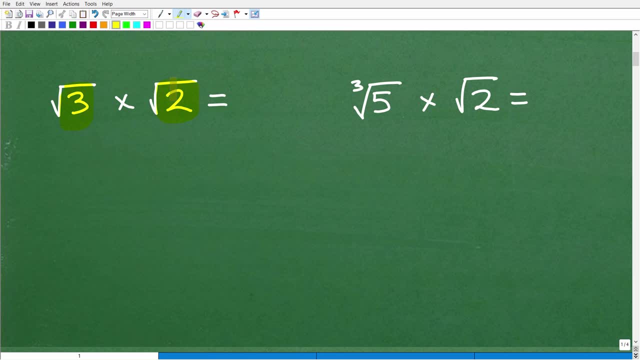 times the square root of two. So how do we multiply Square roots? Well, this is going to be so easy. You're going to be like, wow, I can't believe it's this easy. Well, the square root of three times the square root of two is equal to the square root. 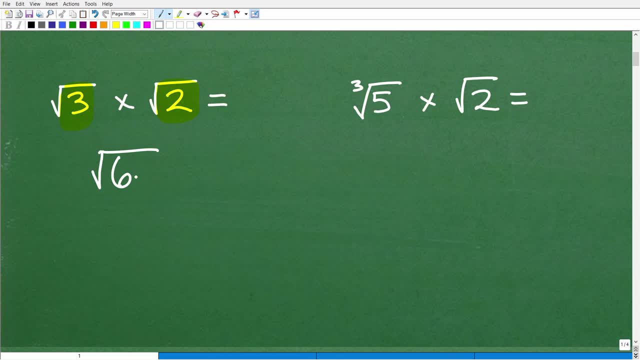 of six. Okay, So square root of three times the square root of two is equal to the square root of six, But why? Well, let me go ahead and show you why. So the square root of three times the square root of two? what we did here is just put one big radical, one big square root symbol And then 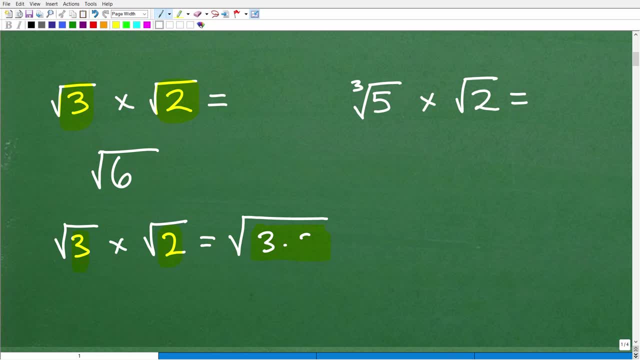 right here. Okay, So this is going to be the square root of three times two. Okay So we have a property in algebra basically looks like this: the square root of A times the square root of B- We can kind of formalize what's going on here- is equal to the square root of A times B. Okay So, 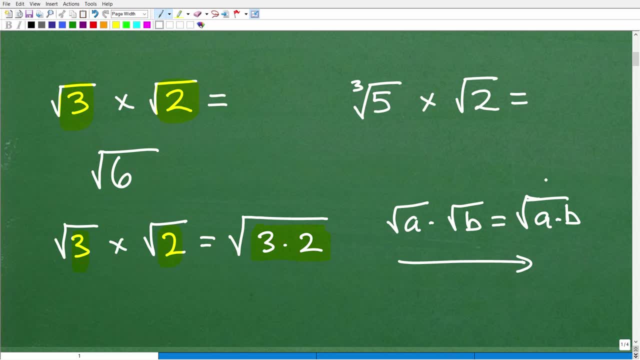 you can kind of think of this property in this direction and it can also think of it in this direction. I'll show you exactly what I'm talking about in just one second. But you know again, algebra and mathematics does not have to be complicated. What happens is something as simple. 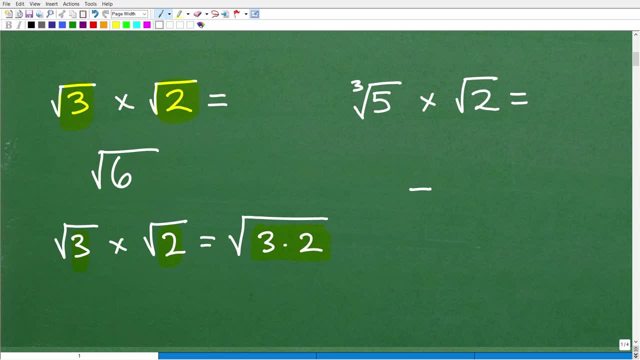 as this. you'll learn a lot of little simple things And you're like, oh, that's easy, That's easy And you just start collecting all these little procedures that are not difficult. But you know, you accumulate a lot of these things And if you're not taking good notes and practicing, 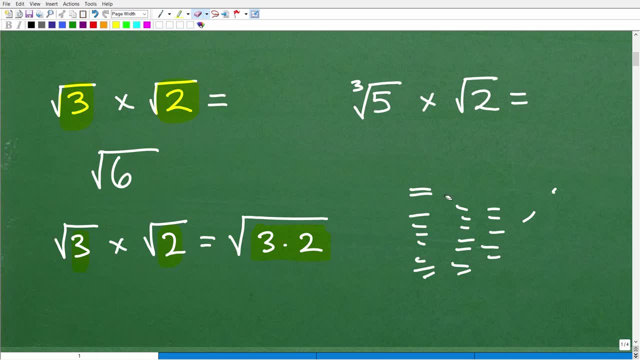 what ends up happening is students get confused. Okay, So just because it's simple and easy doesn't mean that you can't make a mistake, because you can very well forget this stuff if you don't follow through and practice. But look at a problem like this here. Of course, this one is the square root of three times the 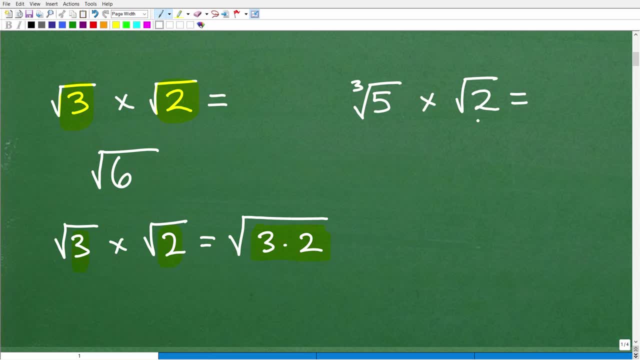 square root of two, And we saw the answer is square root of six. But how about a problem like this? So we have the cube root of five. That's what this is times the square root of two. So what is the answer? Okay, Can we do this problem? Well, the answer is no. we cannot do this problem. 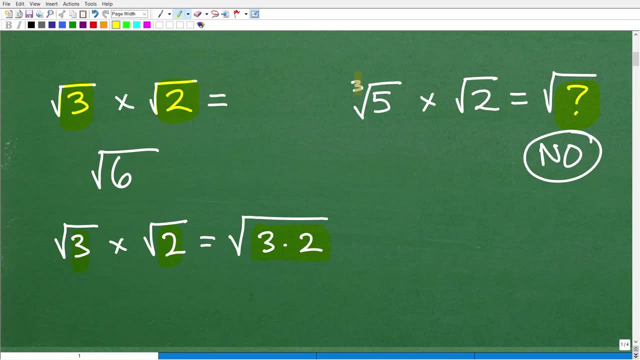 Now, why can't we do this problem? Well, some of you might be thinking: well, does it have something to do with this little thing? right there? You would be absolutely correct. This is the cube root and this is the square root, This little. 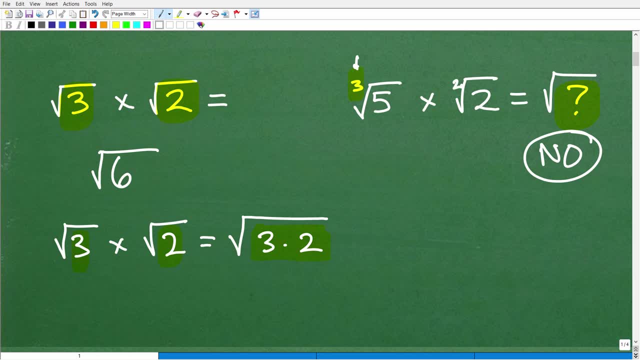 thing is called the index, And right here in the square root there's a little two up there, a little invisible two, And this is for another separate video, but you don't need to really know this here. But here's the thing: These numbers have to be the same, So you can't. 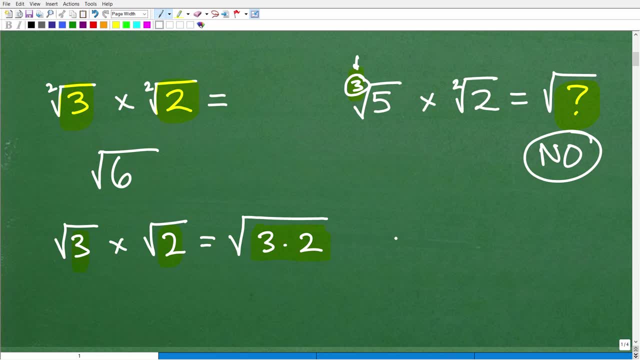 multiply a cube root and a square root. Okay, But if I had the cube root of five and I wanted to multiply by the cube root of two, I would be absolutely correct. This is the cube root and this is the square root of two. Well, guess what? That would be the cube root of 10.. Okay, So you can definitely. 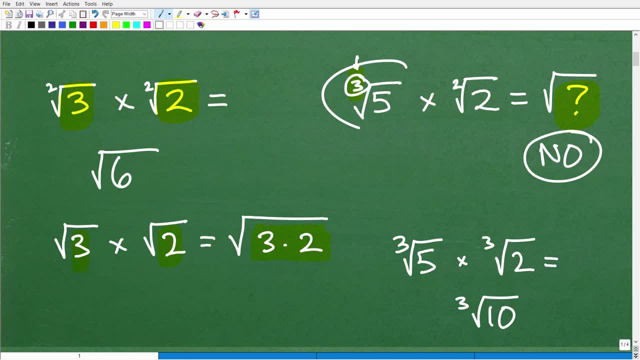 do that. Of course, this video is focused on square roots, but I wanted to make this clear because this is a little bit more. these principles follow through in a broader sense to radicals. Okay, So it doesn't always have to be square roots, But anyways, just wanted to be super. 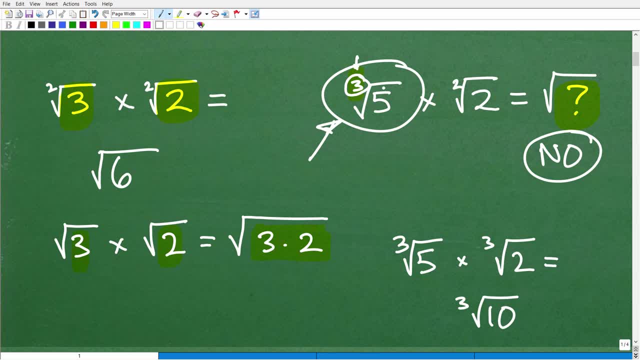 specific about this, because you definitely may see this on one of your algebra quizzes or test. Okay, So that's it. Okay, So we have the square root of five and we have the square root of six. All we need to do is multiply the individual factors underneath one big square root and 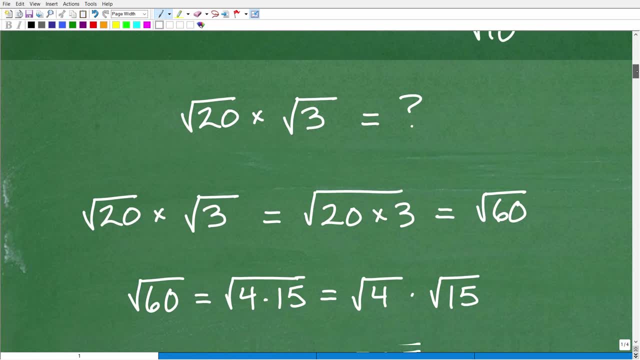 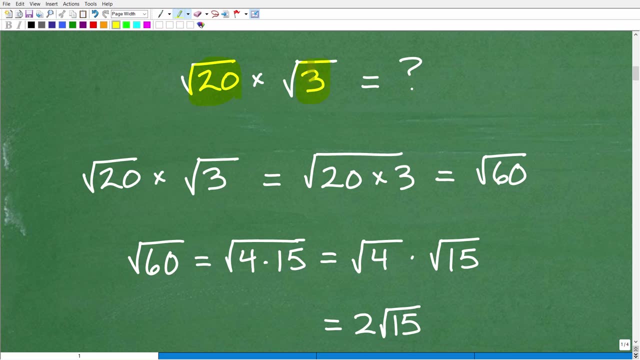 simplify from there. So now let's go back to our original problem and take a look at the square root of 20 times the square root of three. Okay So, square root of 20 times the square root of three. we're just going to put these factors 20 times three underneath the one square root, So that's. 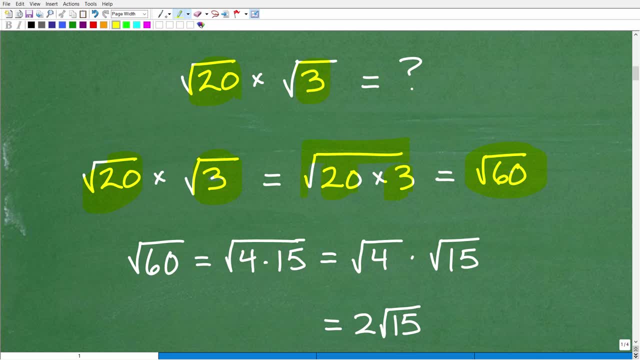 going to be equal to the square root of 60.. Pretty easy stuff, right? So if you got this as you're answer when I asked you in the beginning, if you know how to do this, well then I must go ahead. 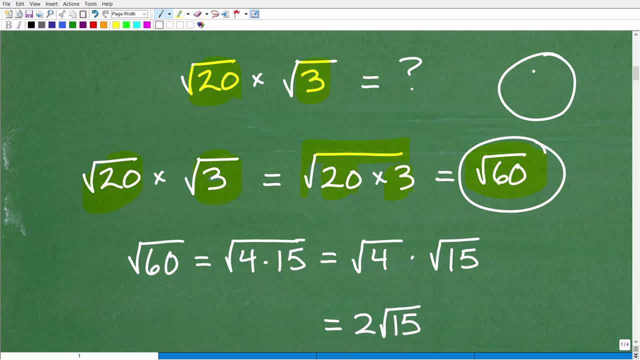 and give you a nice little happy face. Let me fix that happy face up. Here we go. That's a better happy face, Nice job, Okay. However, I would say most teachers may not give you full credit for this answer. Okay, For me, because I'm a nice teacher, I'd probably give you full credit. 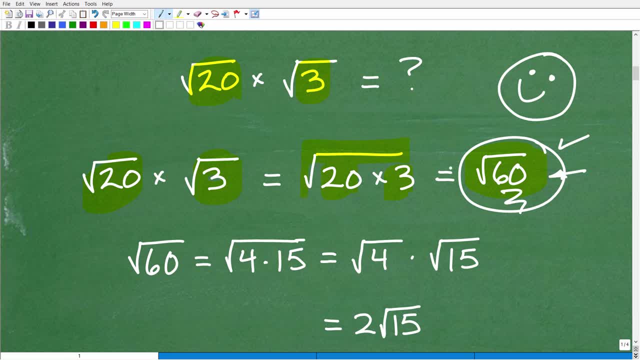 but I would give you a little bit of a warning And I would say: listen, you need to simplify your final, final answers, And I'm actually going to be posting another separate video on this, on how to simplify square roots So effectively. this is like getting a a fraction problem correct And let's say: 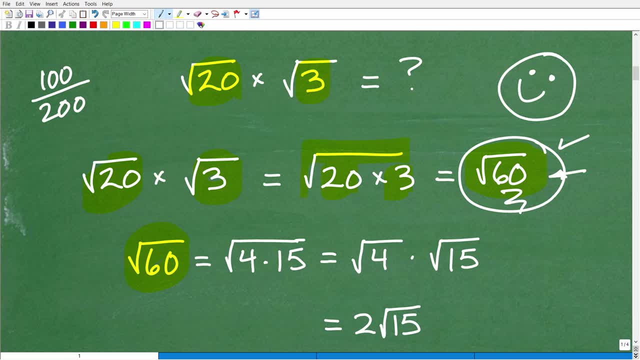 your final answer was 100 over 200. Okay, Now, although that would be your final answer, let's say that's correct, Technically correct. Your teacher would probably get you know upset at you if you didn't reduce your 100 over 200 to one half. Okay, So let's just 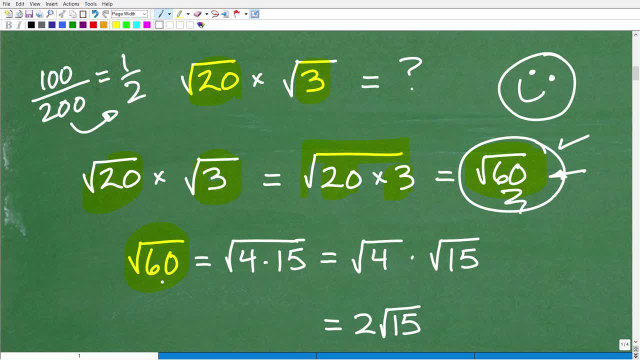 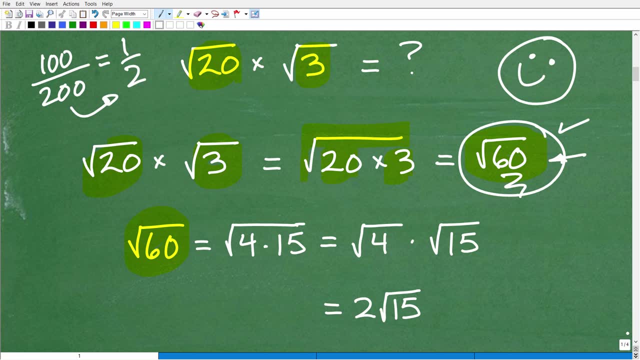 same thing with the square, uh, with square roots, and uh, the square root is 60.. We can actually simplify it, And you're going to need to know how to simplify square roots. Of course, we're talking about how to multiply square roots, but let's just take a look, quick look. 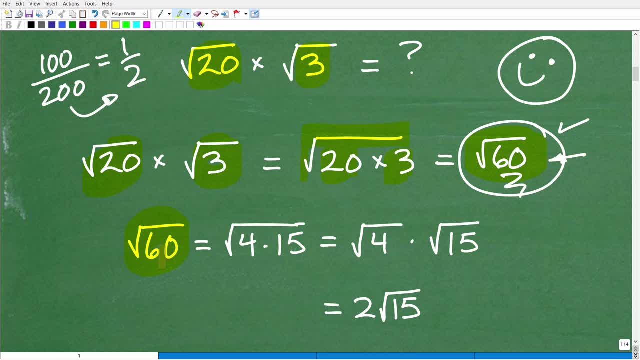 on how to do this. So the square root is 60.. Okay, We can actually go uh kind of pull this apart, Okay, Like in other words, undo this problem, but this time I'm going to think of 60 as four times. 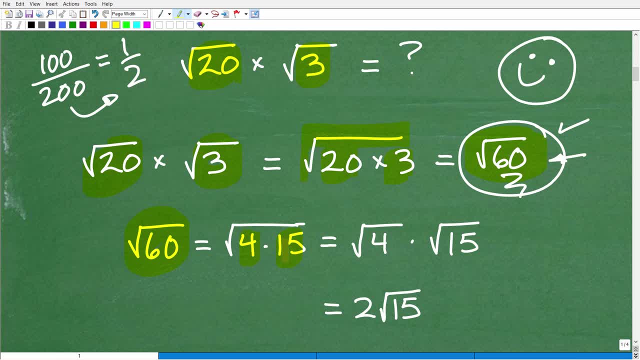 15.. Okay, So I'm kind of, uh, going to be factoring this number. So the square root of 60, is the same thing as a square root of four times five, And now I can have break this up into two. 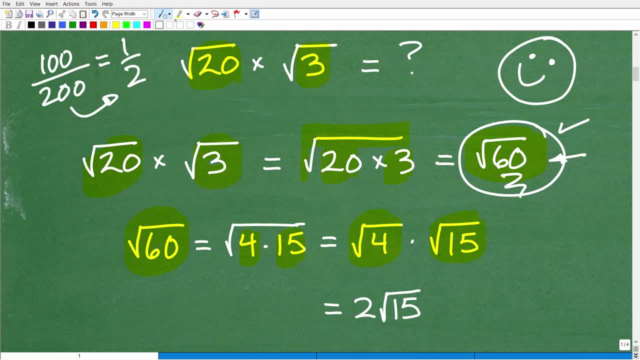 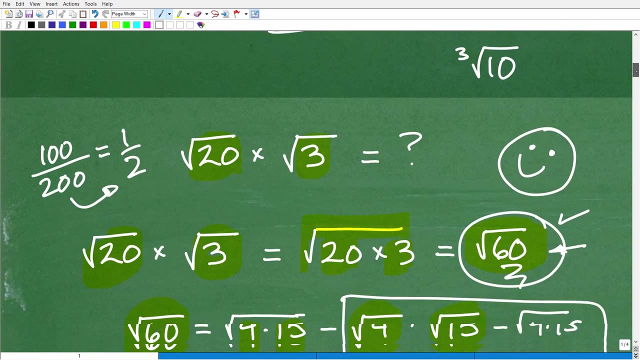 separate square roots, a square root of four times a square root of five. If I asked you to do this problem right here, you would say: Oh, that's the square root of four times 15, which, of course, is the square root of 60.. Okay, So remember, as I stated back over here: uh, Oh, I'm sorry about. 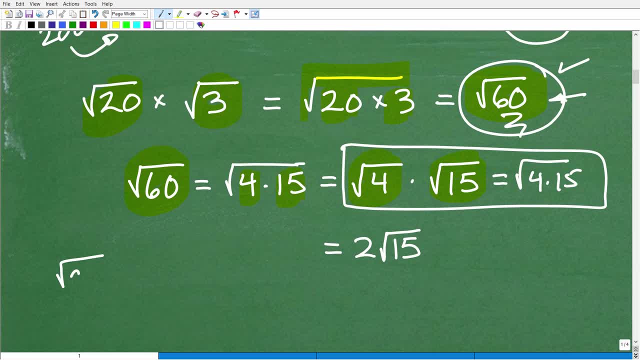 that I erased it, but let's take a look at this property again. That's the square root of a times B is equal to the square root of 60.. Okay, So let's take a look at this property again. That's the. 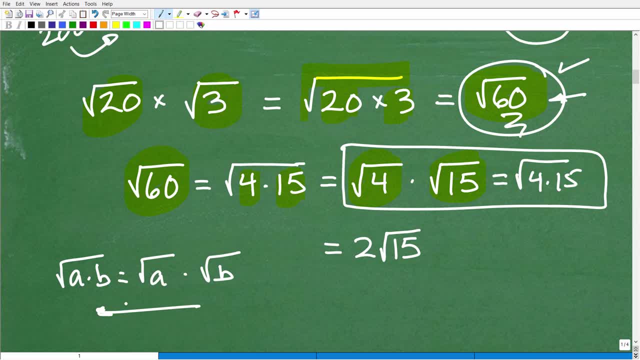 square root of a times the square root of B, So the property works in both directions. Okay, So I can- um, I can, separate the factors here. So just to be crystal clear about that, you want to uh see how multiplication we're multiplying two square roots. You can also break it up and uh. 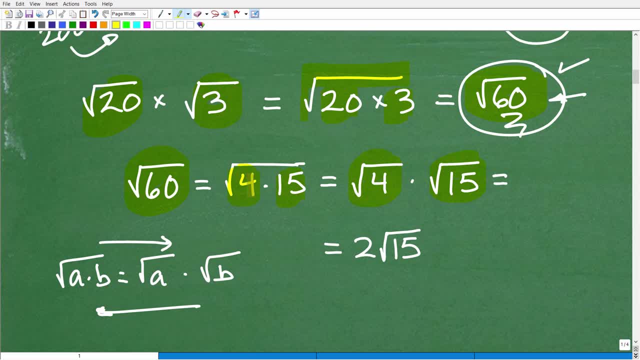 write that in terms of its respective factors. Now, I like the square root of four, because I can find the square root of four. This is what we call a perfect square, because the square root of four is two. Okay, So that's now two times the square root of 15, not the square root of four times the square root of. 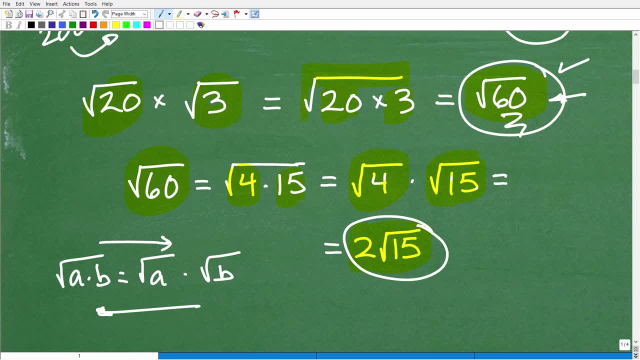 15.. So your final answer would be two times the square root of 15.. This is the most simplified version of this. Okay, So, um, again, we're focused on how- uh, multiplying square roots, but you want to also know how to simplify square roots as well, because you know all this stuff. 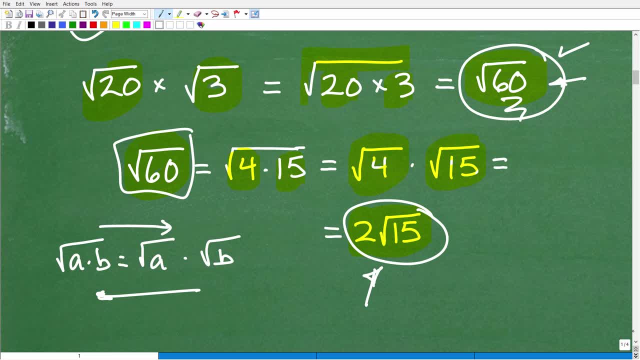 is connected, Okay, So when you're learning about square roots, you're going to have to learn how to divide square roots. multiply square roots, add, subtract. simplify that stuff as well, So follow through. If you didn't know that the square root of 16 is equal, 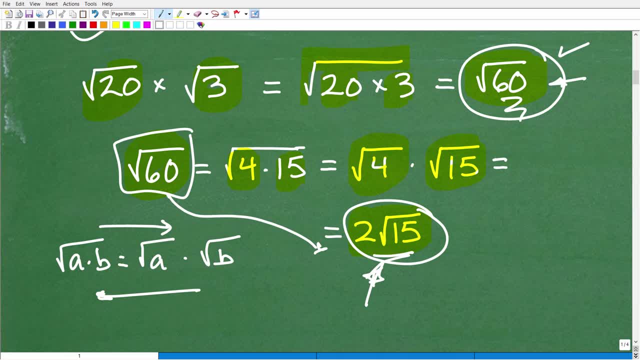 to this. now you know all right, But if you got this as your final answer, then I must upgrade your nice little happy face with a good old 1981 Mohawk haircut. I grew up in Southern California, by the way, So I saw all kinds of crazy haircuts: uh out there and um, uh, hairstyles and whatnot. 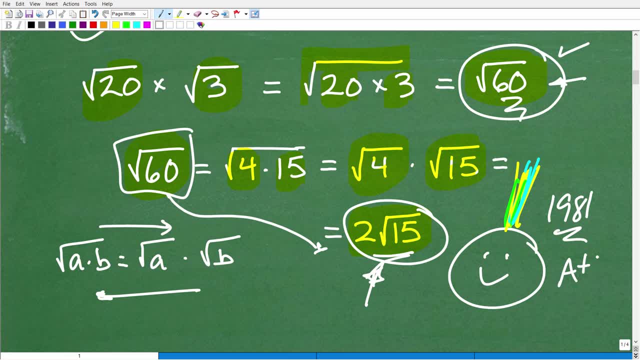 but that was an impressive haircut, Just like your. well, I don't even know if it's a haircut right, It's really taking your hair And standing straight up with a lot of hairspray, which was a pretty impressive feat in and of. 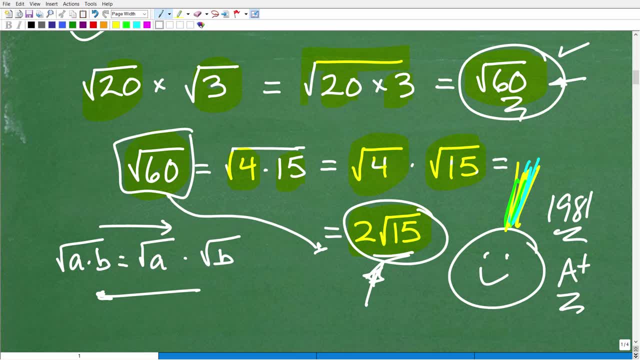 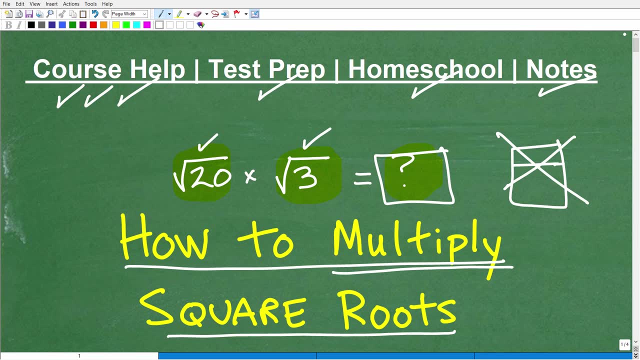 itself. But anyways, if you got this all right, then that's just as impressive as well. So nice job. but here's the deal. Um, if you didn't know how to do this, well, now you got a good introduction. Okay, Don't look at this as an end. all be all lesson You want to follow through. 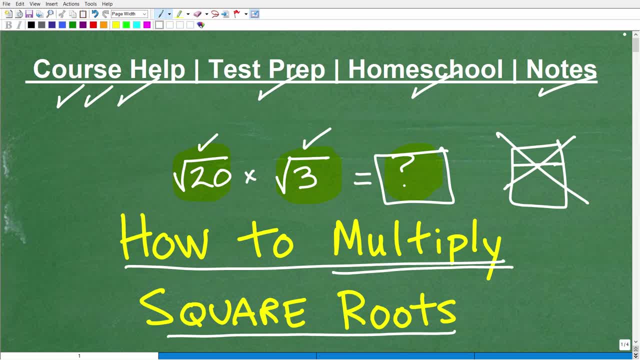 and maybe take a look at some of my uh, more formal instruction, uh, in any one of my algebra courses to really master this. But I do have additional videos on my YouTube channel, but if this particular little video helps you out, we'll go ahead and consider smashing.